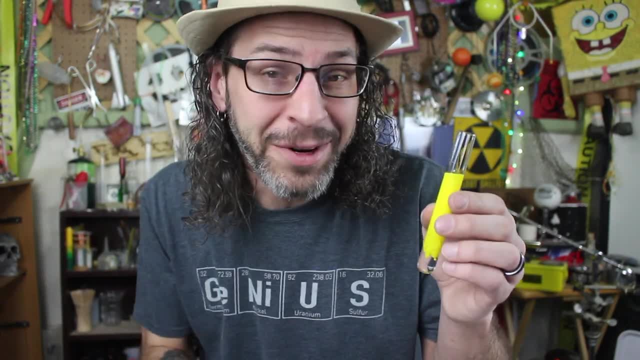 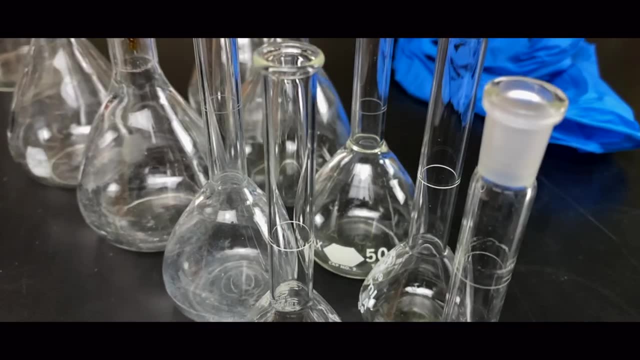 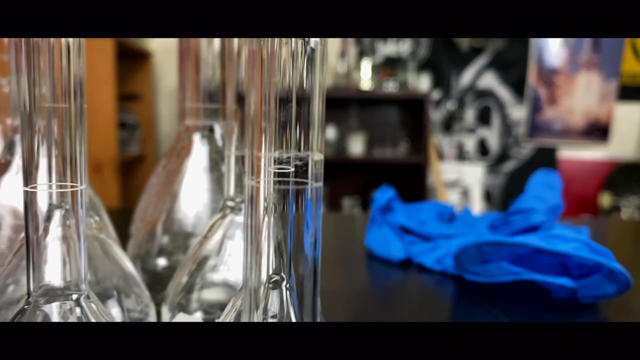 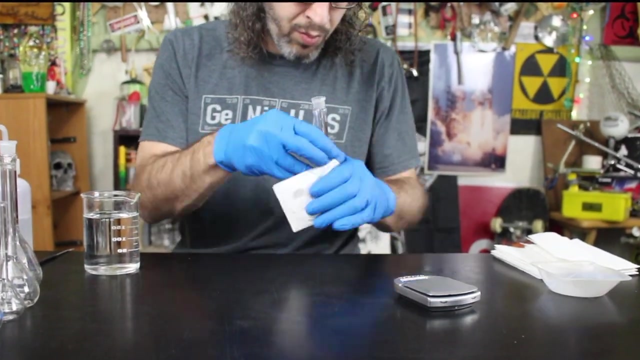 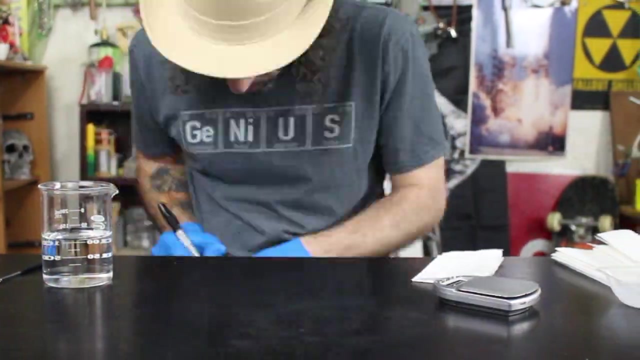 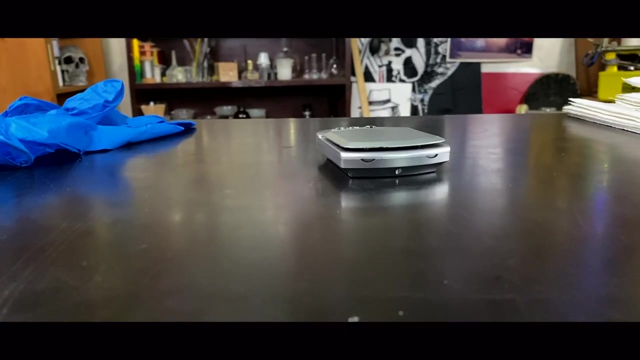 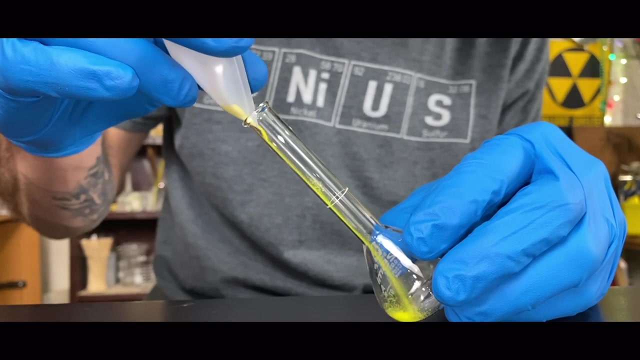 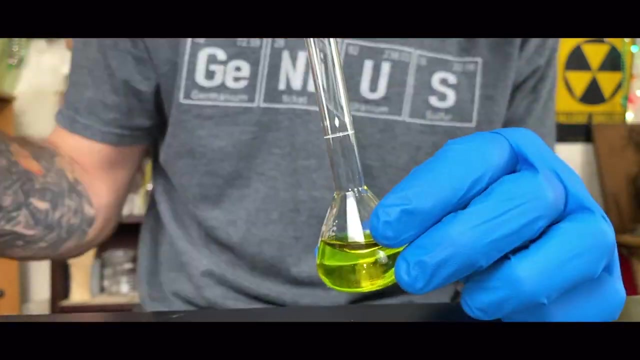 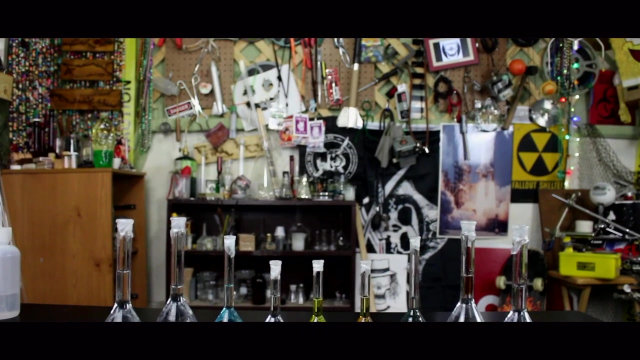 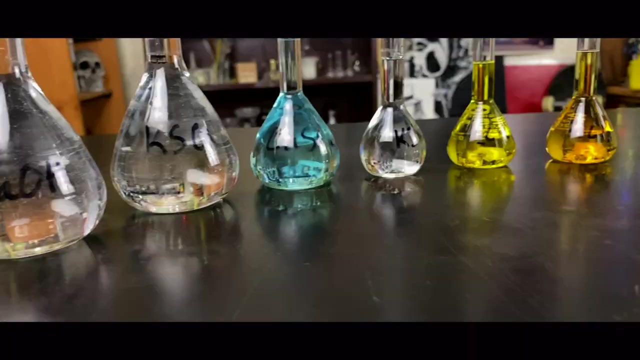 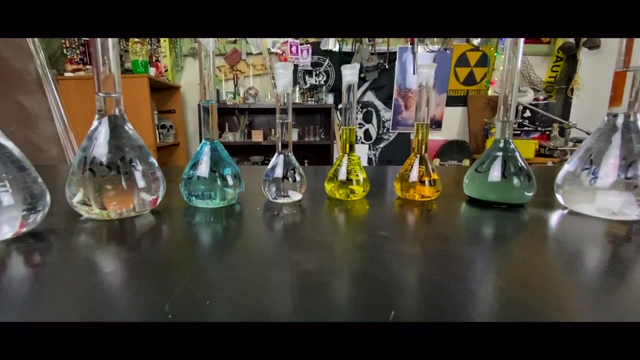 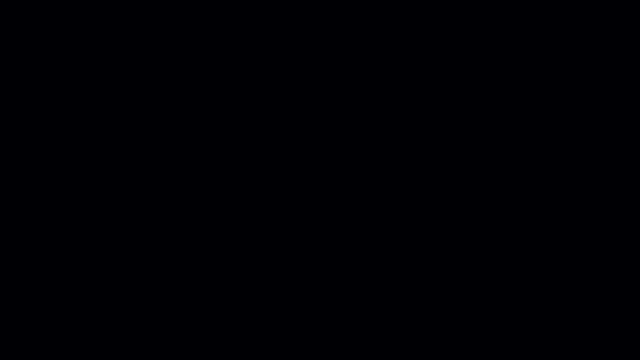 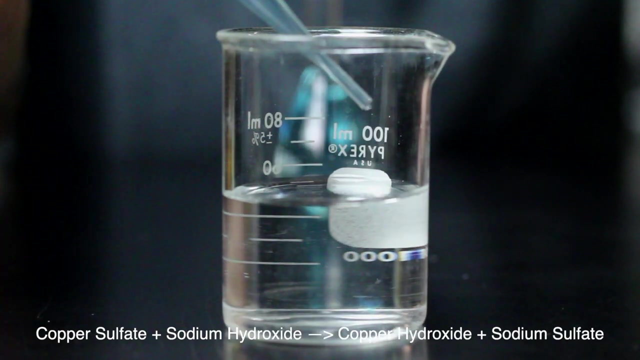 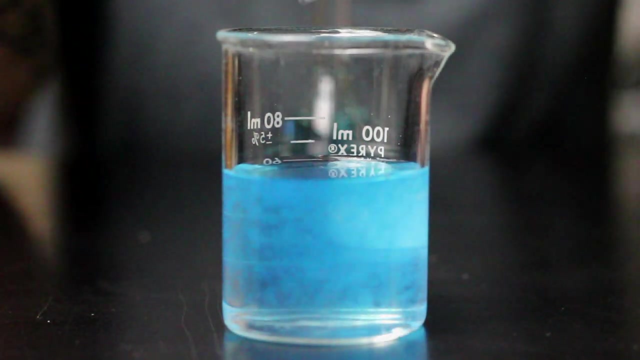 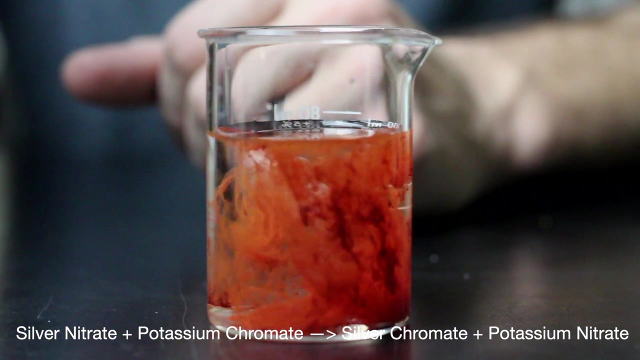 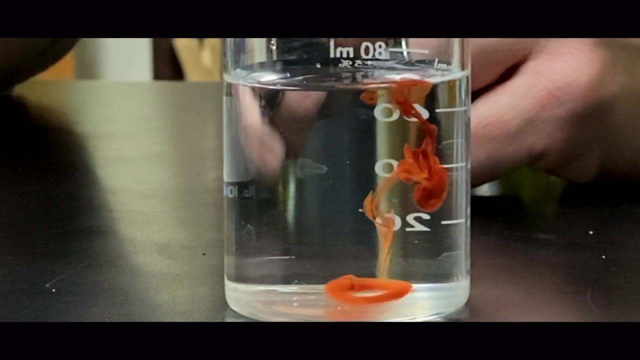 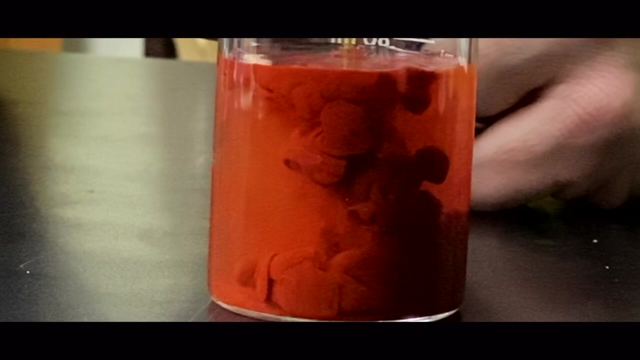 Created, Creating an insoluble solid that falls or precipitates to the bottom. Thud, Thud, Thud, Thud, Thud, eccalge Name: Trepidation: Tile menu. Enclosure menu. Thank you, Thank you. 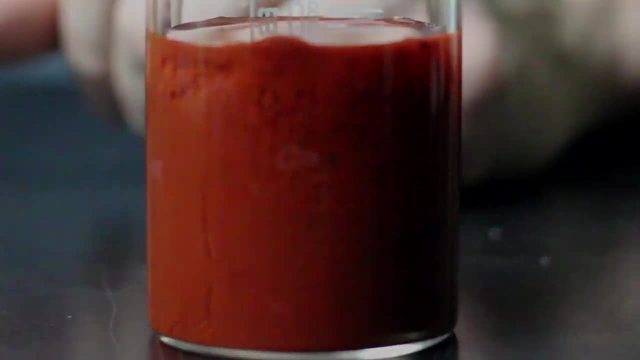 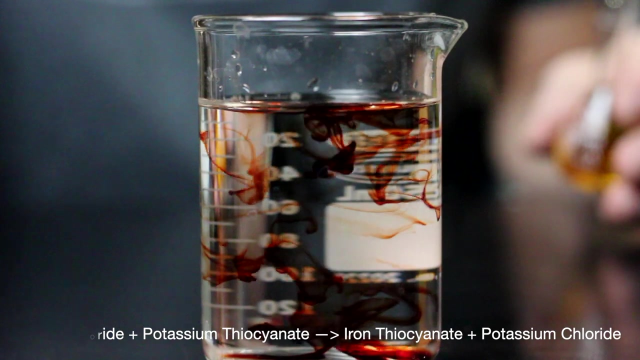 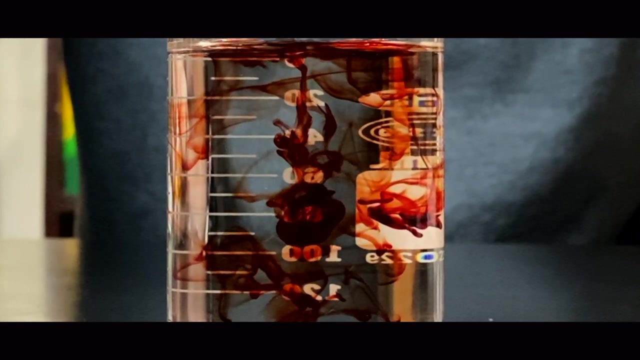 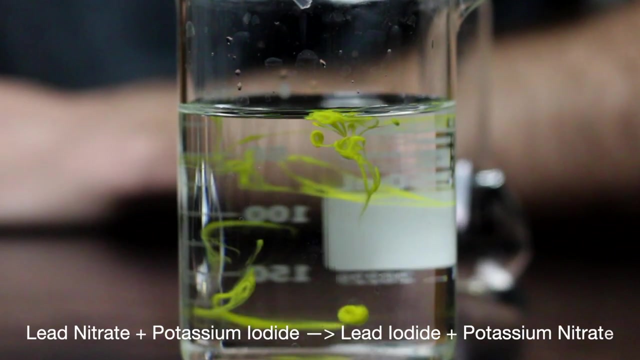 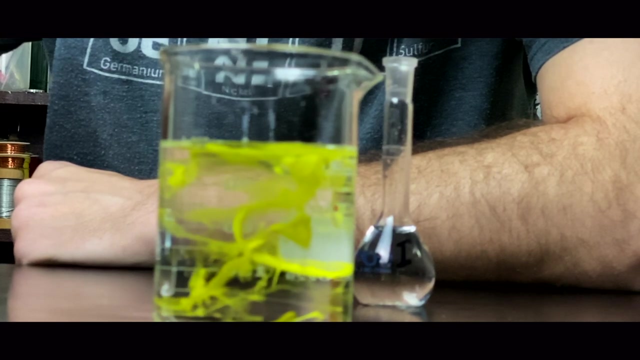 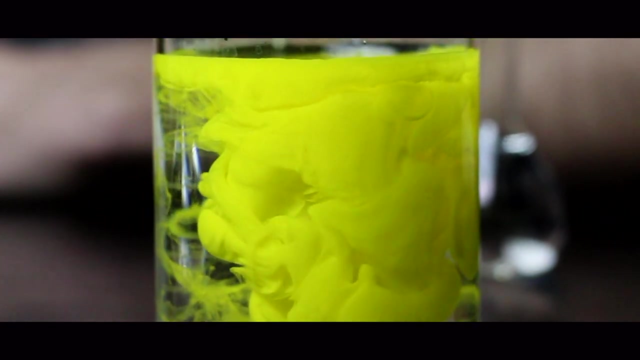 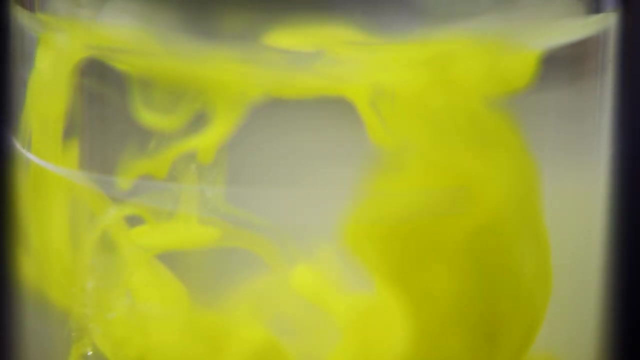 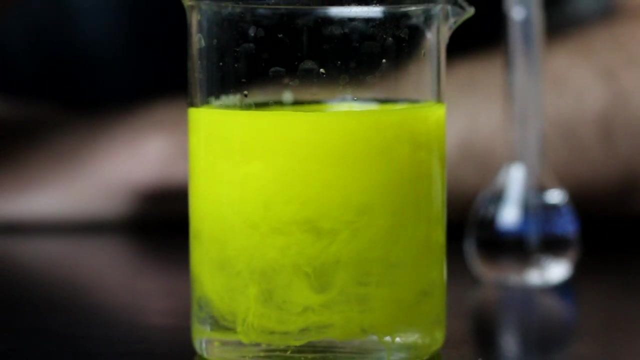 Thank you. The solutions are made using water as the medium for dissolving ionic compounds such as salt, sodium chloride or silver nitrate and potassium thiocyanate. When the solutions are mixed, the ions exchange partners like two couples on the dance floor, resulting in two new